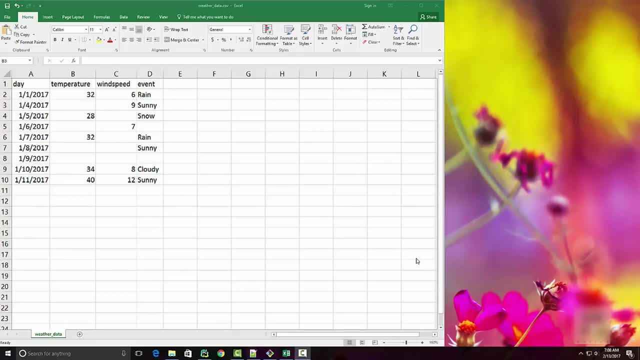 Dear friends, in this tutorial we are going to look at how to handle missing data in pandas. Now, often when you are downloading data from internet, or, let's say, getting it from any other source, it might have missing values, as shown in this CSV file. This file contains New York City's weather data and you can see. 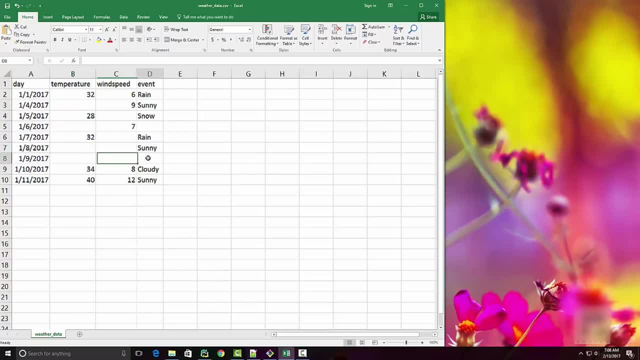 that some of these cells are not having any value in it. Also, it is missing the data for 2nd and 3rd January. Okay, so when you're processing this kind of information in pandas, we will see how you can deal with these missing values. 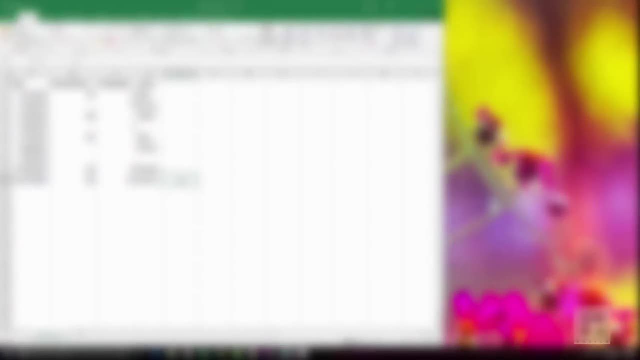 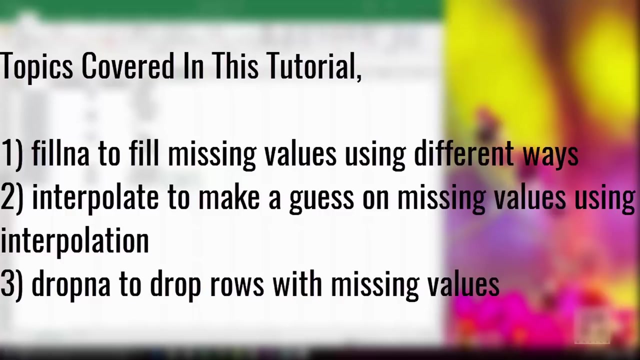 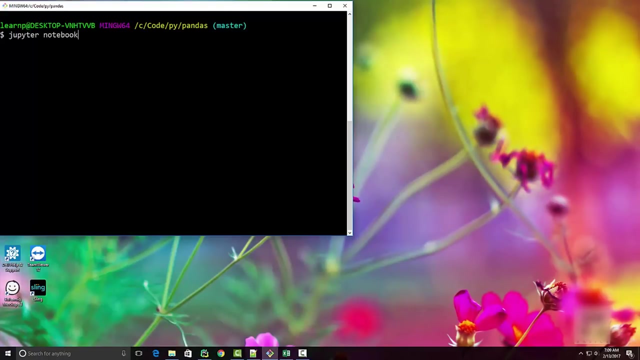 using fill any, interpolate and drop any methods. I have more tutorials on how to handle missing data, but this is just to start and we are only covering these three methods. Okay, so, as usual, I am going to start my Jupyter notebook Now. if you don't know what is Jupyter notebook, I have a separate. 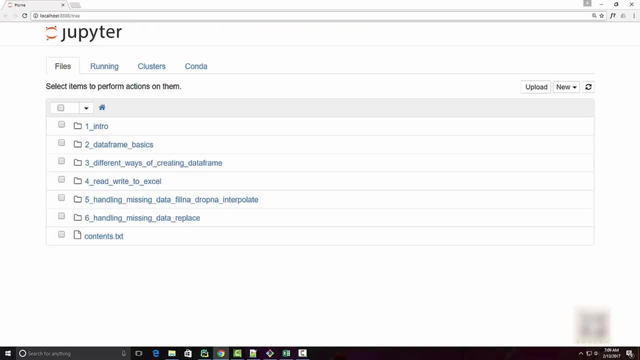 tutorial on it, but you can also use any IDE of your choice, such as pycharm or not. pay plus, plus, whatever you prefer. I like Jupyter notebook because it is great with data visualization. Okay, so I'm going to click on new and start a. 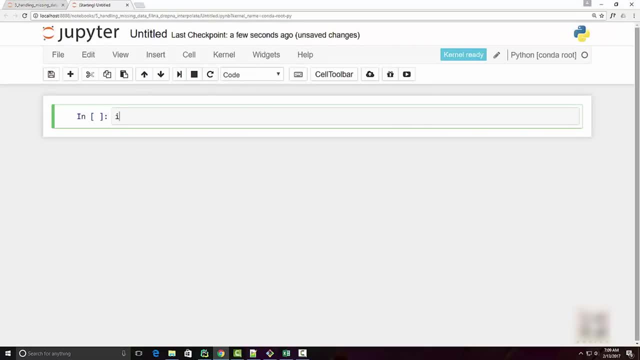 new Python notebook, and the first thing we do is we are going to create a new Python notebook. So what I am going to do, as usual, is import pandas as PD and then I will read the CSV file that I just showed you, Okay, and print the data frame, The star. 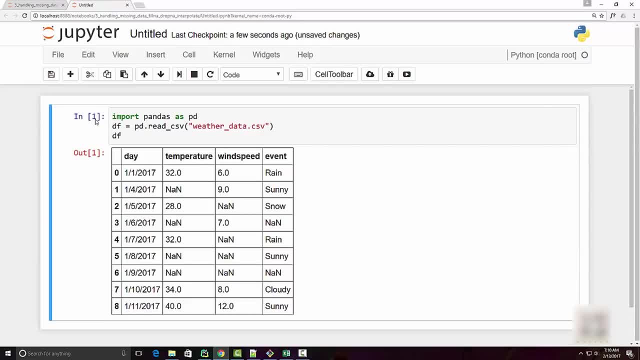 that you are seeing here means it was processing it, so it read this CSV file successfully into a data frame. Now, for the purpose of this video, I am going to this tutorial. I want to make my day a date column, so let me show you what I 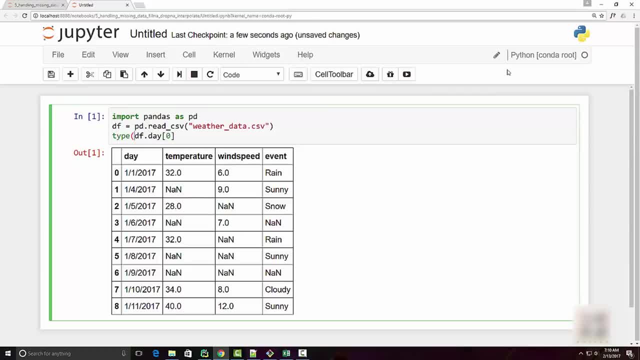 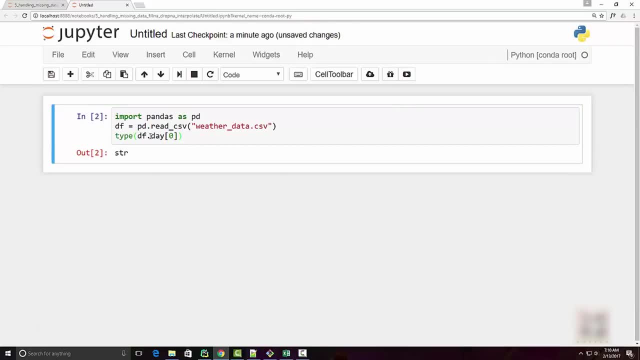 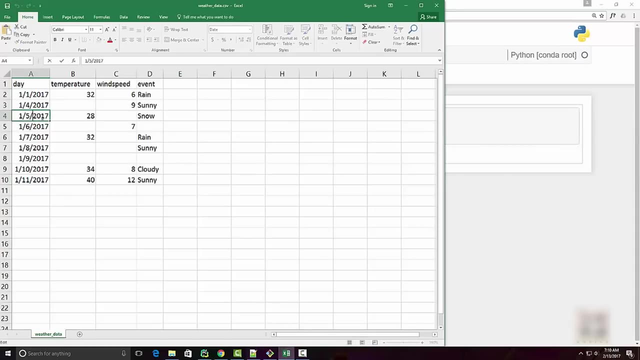 mean by that. so when I, when you normally read CSV like this, what what it's gonna do is it's gonna read day as a string column, you can see it is a string. so whatever you're seeing here, this is nothing but but a string. it's not an. 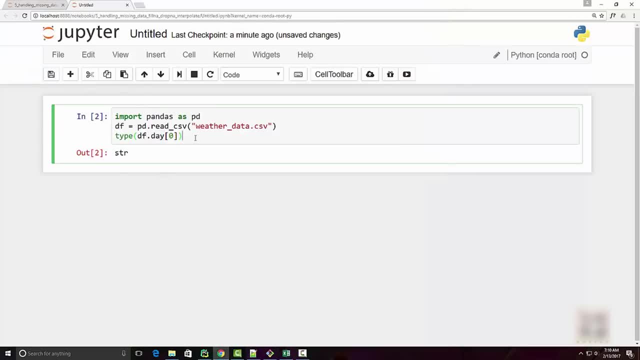 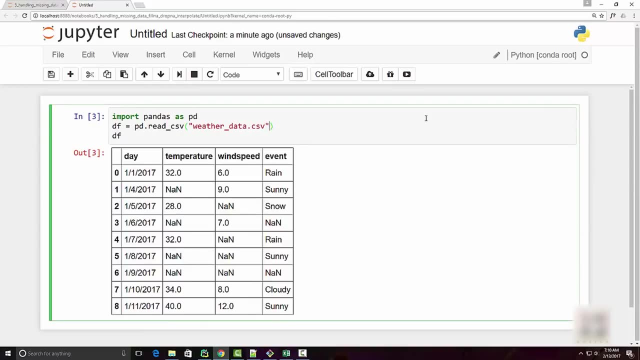 excel file. okay, it's a CSV file, so I want to first convert that column into a date column, and for doing that you have to use pass dates argument and in that you can say that pass day column as a date type. okay, and when you do that 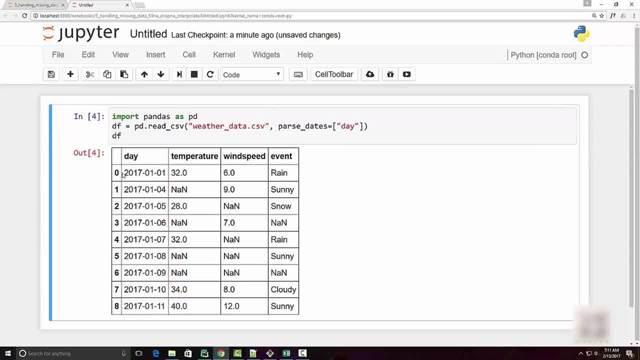 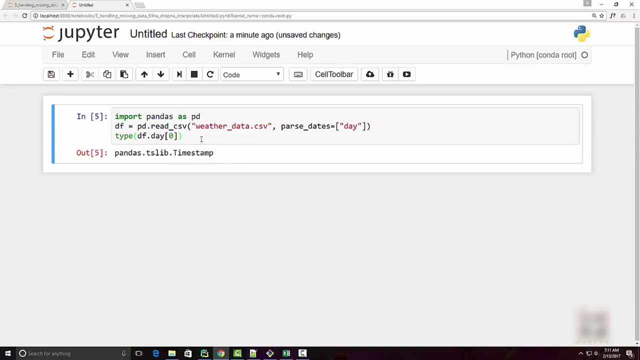 okay, let's Okay, let's see. first print it. you can see that it converted. now, by looking at it you cannot probably figure out the type, so what I do usually is: just so you can see that now the type is timestamp. okay, so we're good, all right, so I got day as a 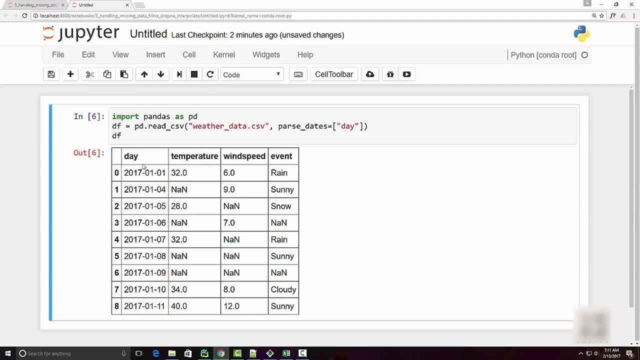 date time column. now I want to make this an index for my data frame and it's, and in order to do that, you can just say DF dot set index day as your index and in place equal to true. remember you have to do in place equal to true, otherwise it's. 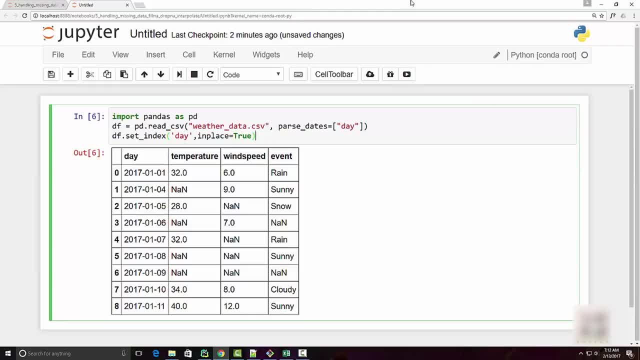 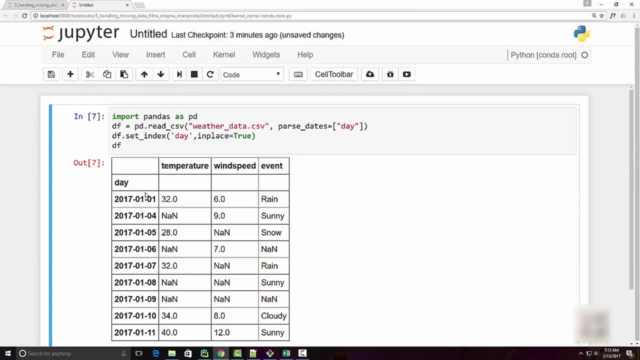 not gonna modify the original data frame, but instead it will return a new data frame. okay, and when you do that, you got day as your index. now if you have NA values and if you are processing this information, then you have to do spatial handling. you have, like, if value equal to any, then do this special thing. okay, often it makes sense. 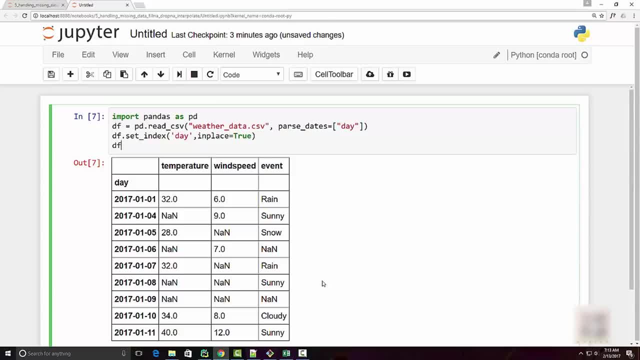 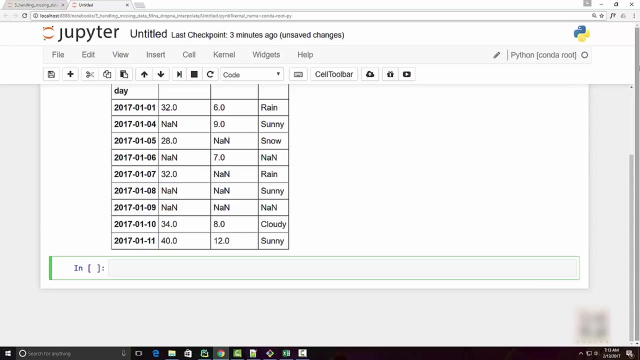 to replace these any values with some meaningful value or a guess. okay. so in this case, let's say, I want to replace all any n values with some other value. okay, so the first method that we are going to cover is fill any okay. so what you can do is DF dot, fill any okay, and in bracket you can pass the value that. 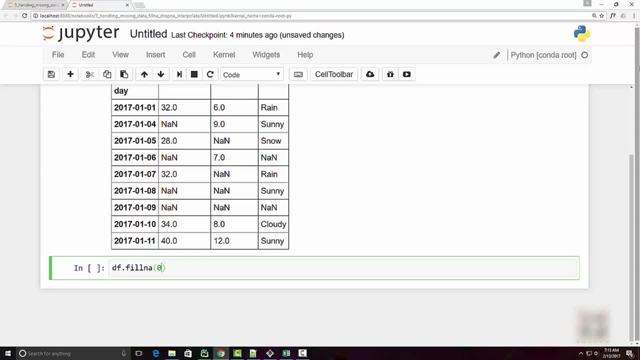 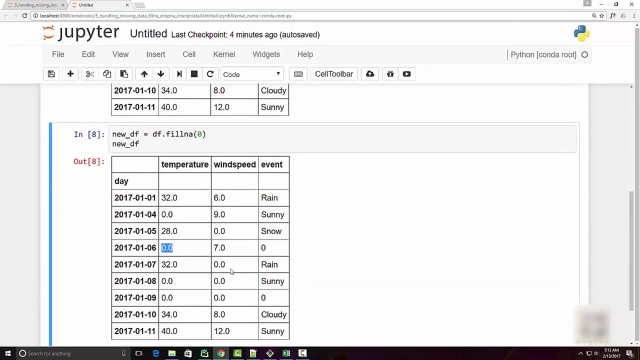 you want any to replace with, okay, and I'm not going to modify my original data frame, but instead back into a new data frame. and when I run it, you can see that all these nn values that it had, it replaced them with zero value. you can see that everything. 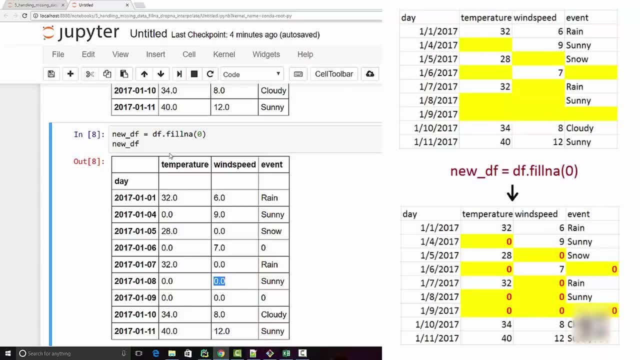 is everything that was any is zero now. okay, so this is good. now, sometimes having zero is not probably the best guess, so you want to come up with any values that you want to replace with some other value. okay, so this is good. now, sometimes having zero is not probably the best guess, so you want to come up with. 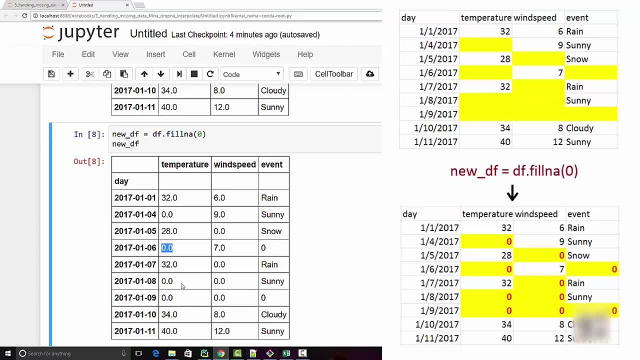 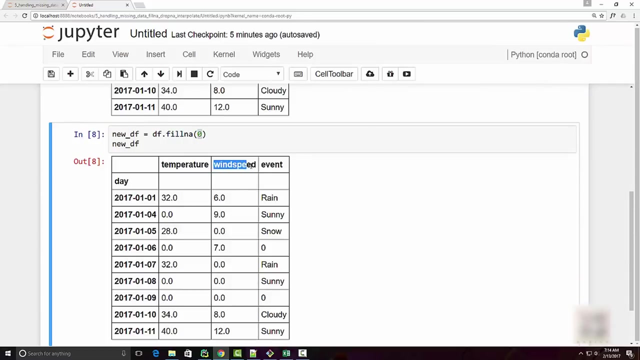 with a better guess, okay. for example here, in the case of event, what does zero mean? right? so maybe you want to use fill any, but you don't want to fill entire data frame with this value. maybe you want to specify different values for different columns? okay, so pandas supports that also. 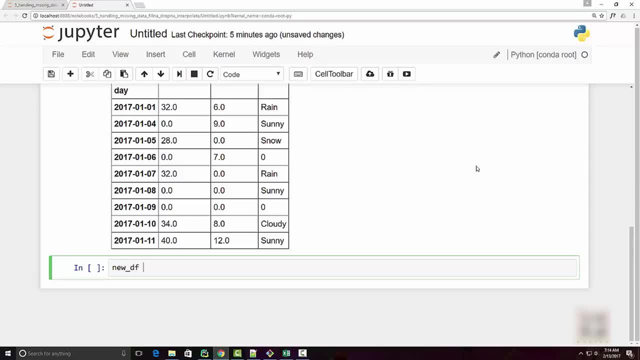 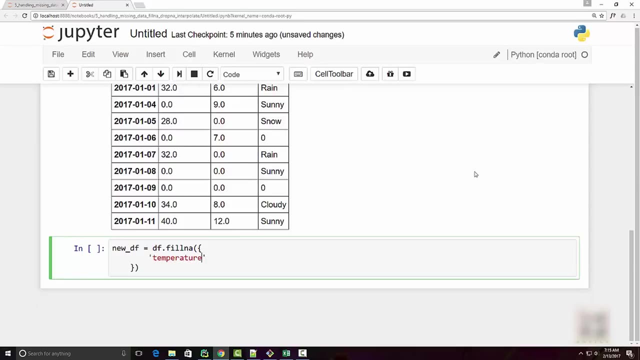 so the way you do it is again. I'm going to receive it in new data frame and inside fill any method. now you can pass a dictionary. okay, now, what does this dictionary contain? so dictionary contains name of the column. okay, now, in temperature column, let's say I want to replace all any values with zero and in 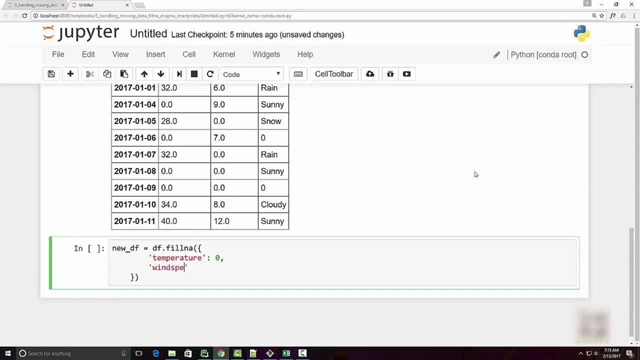 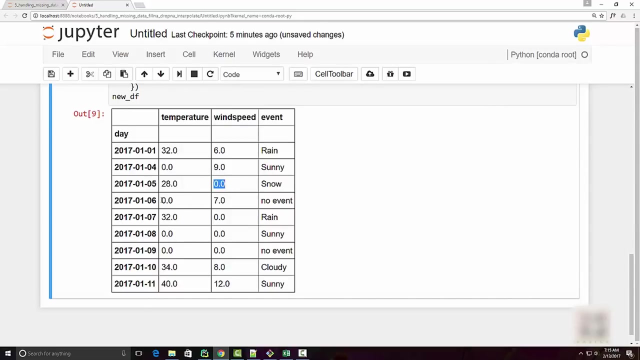 my day, not day, but wind speed column. I want to replace it with again zero, but my event. I want to say no event okay, and then print new data frame now, as you can see here, the temperature and wind speed. it replaced with zero, as you can see here, but the event. now I have no. 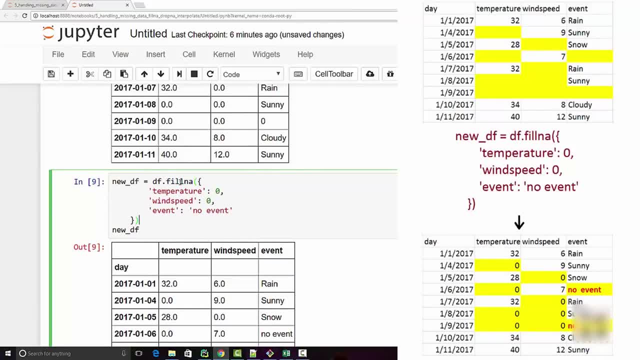 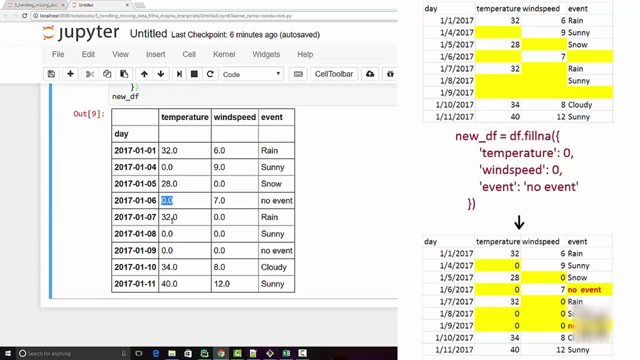 event. okay, so you can just use this dictionary to fill specific values for a specific column, but still I am not happy with how I handle missing values here. because see, if you're calculating a mean or something for this temperature, then mean is gonna come really horrible and if someone looks at data he will think: okay. 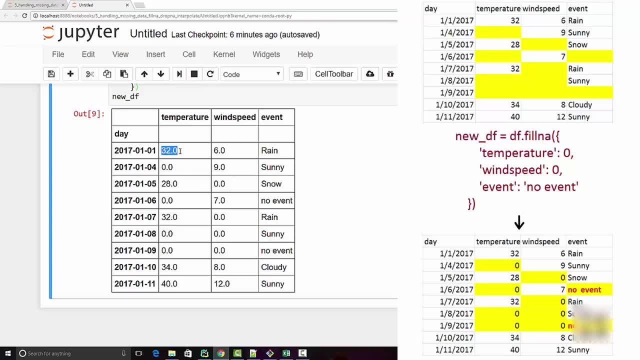 on first January it were it was 32 temperature and the 2nd January it was zero Fahrenheit. right some someone might think this. the went down by so much, but in reality we actually don't know what was the temperature and all we are trying to do is come up with some estimate, okay, so 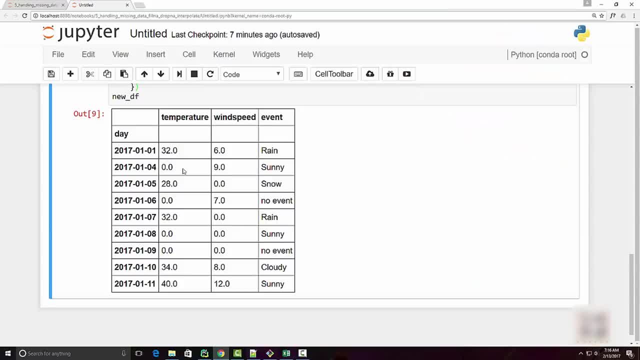 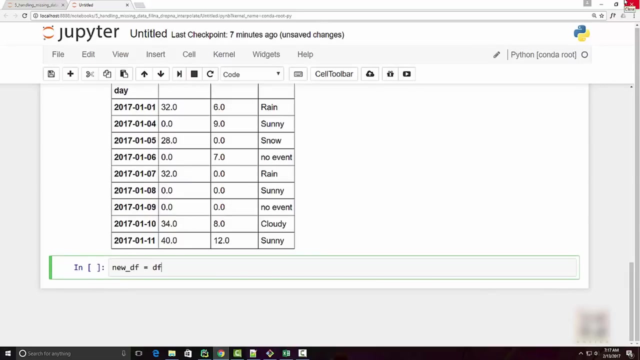 then the other way of getting better estimate would be just to carry forward the temperature on for January here. okay, so whatever was the temperature on the previous day, you carry forward and you do it in a similar way for other two data types. okay, so for that you can use again your fill, any method. okay, but here what? 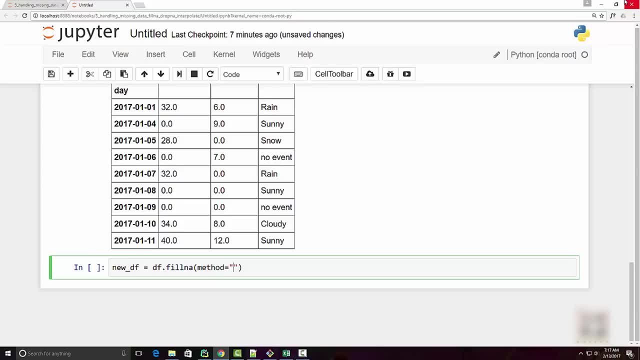 you will do is you will say: method equal to forward fill. forward fill. you can specify by typing F fill. a fill means if I have any value, then just carry forward previous day's value. okay, so let's print that. okay. cool, now you can see that it just carry forwarded the value from the 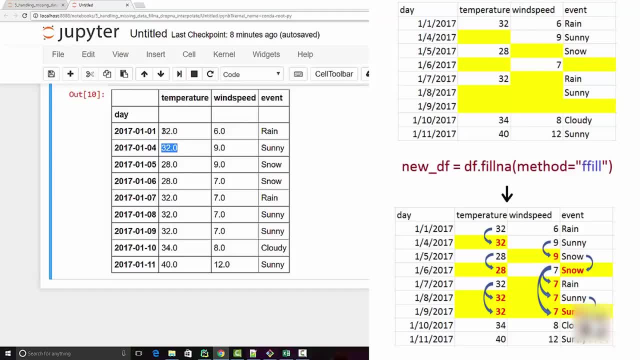 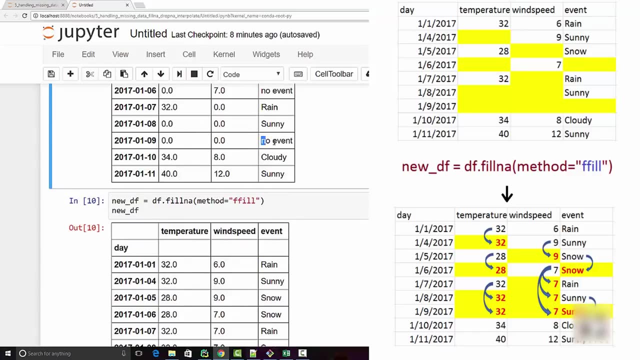 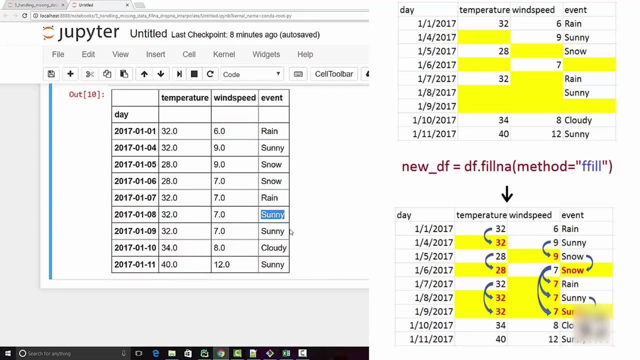 previous day. so fourth January had any value, but now it carry forwarded first January's value here, so this looks little better than just having zero value. okay, same thing on 9th January I, I didn't have any event. so you look at 9 January, now it is sunny because you carry forward previous day's. 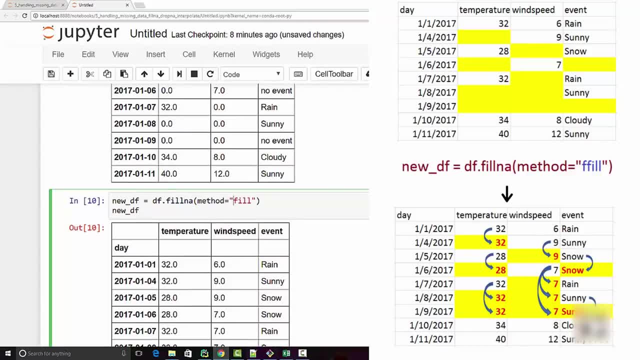 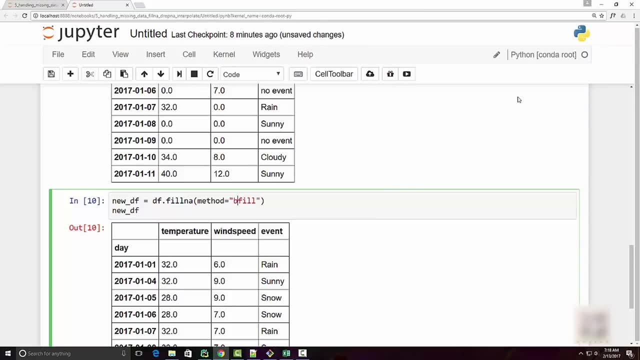 value. you can also use backward fill, meaning carry forward next day's value. it's not really carry forward, but you're copying. instead of copying previous day's value, you're copying next day's value. so if you do that, what's going to happen is now: 4 January has a value from 5th. 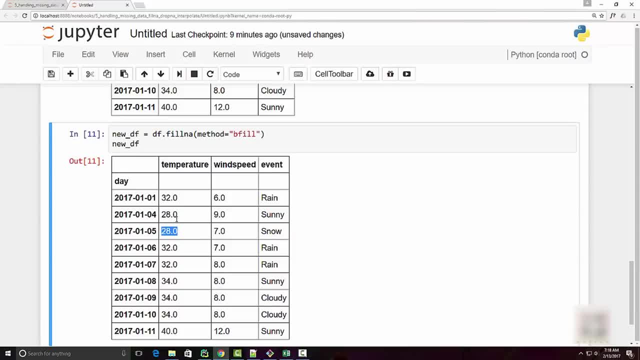 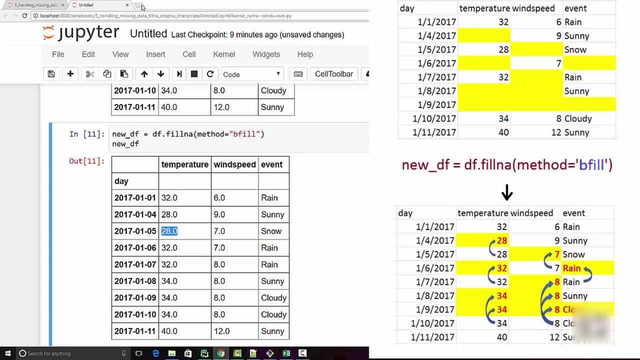 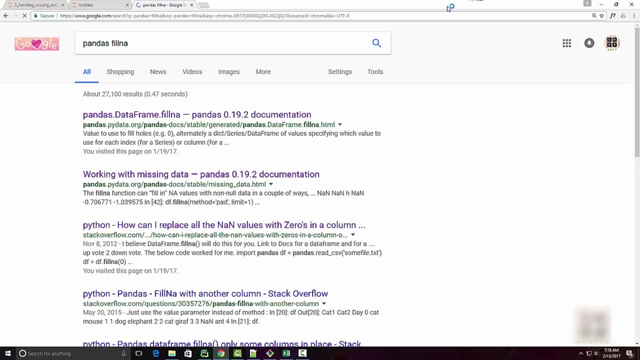 January. so now it copied value from fifth to fourth. okay, so you can use be fill method also. now, if you go to plan does documentation? you can just google in pandas fill any is going to show the documentation for fill any and you can see that we have. 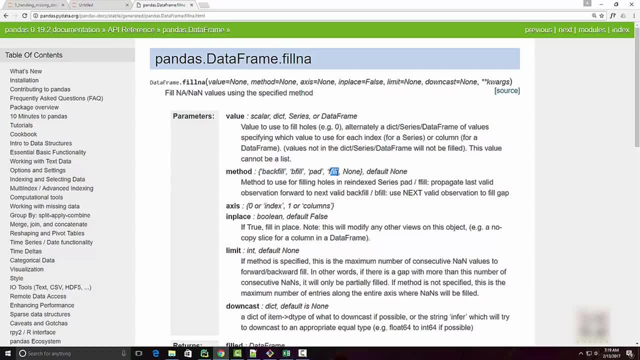 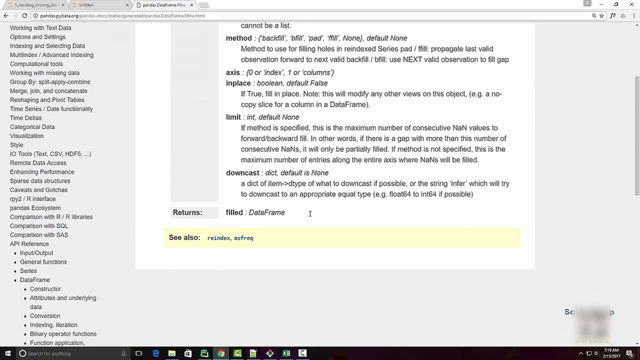 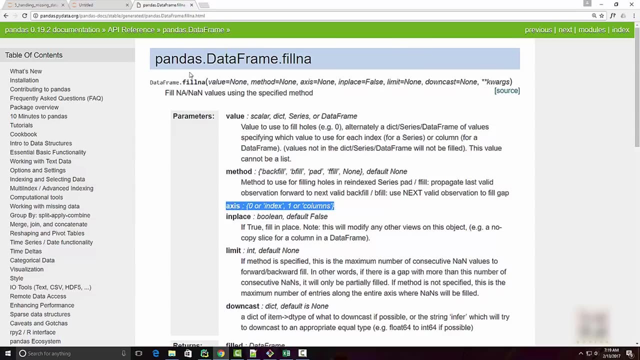 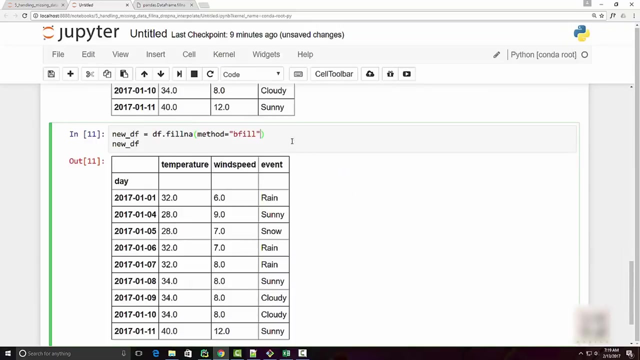 used backfill, B fill and a fill. you can also use pad or blackboard backfill- okay, so you can use all of that. you also have this other argument called axis, so let's see what axes can do for us. so here, if I say X's okay, X is equal to columns. bye. 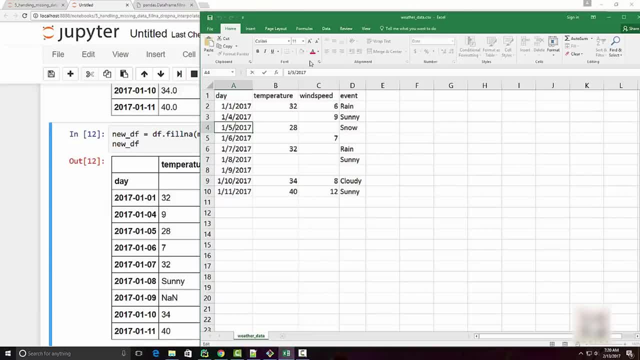 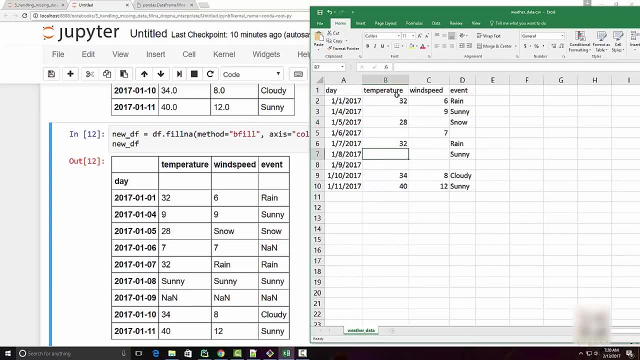 do X is equal to column. what it is doing now is: let me open the CSV file here. so here: previously, when we are using column. what it is doing now is: let me open the CSV file here, so here: previously, when we were using backfill, it was copying values vertically. like it will go vertically and 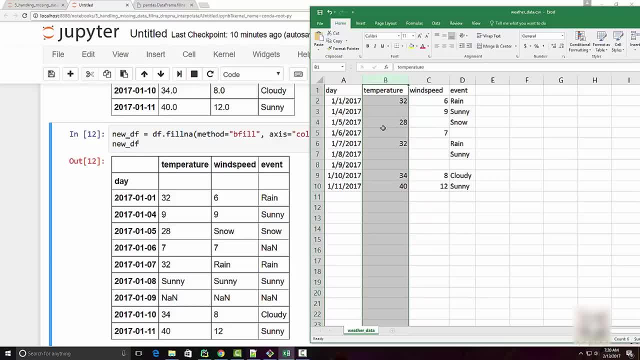 copy value from here to here. but now with X is equal to columns, it's copying values horizontally, so it's going row by row and copying value from previous cell. so here, look at here it's. it was 9 here and it copied that 9 into temperature, so 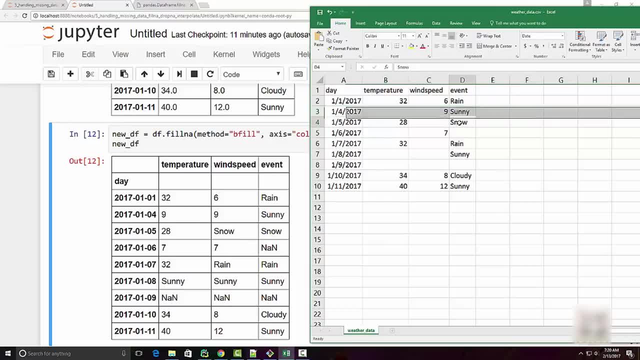 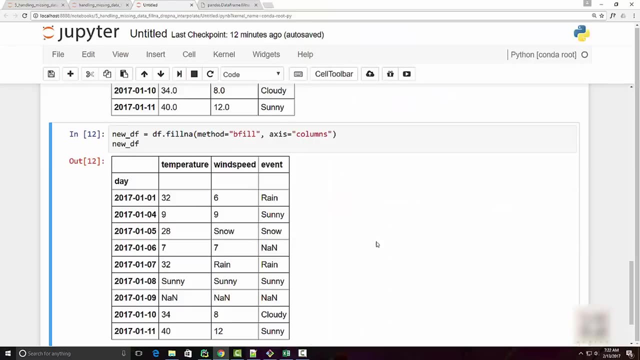 you can see this 9 is copied here. then the snow was copied here, so you can see this was snow and this is also snow now. so you can, based on what kind of data you are dealing with. you can copy it either horizontally or vertically. okay, now if you check the documentation of fill n a, it has another interesting 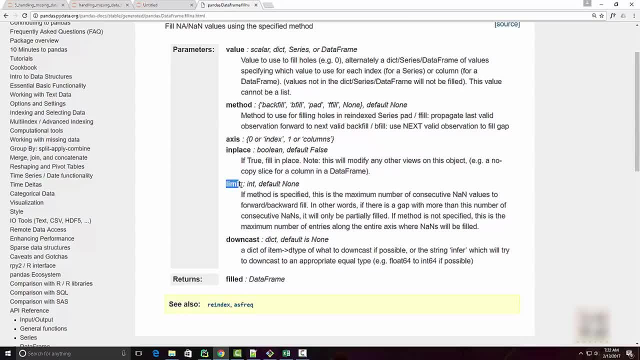 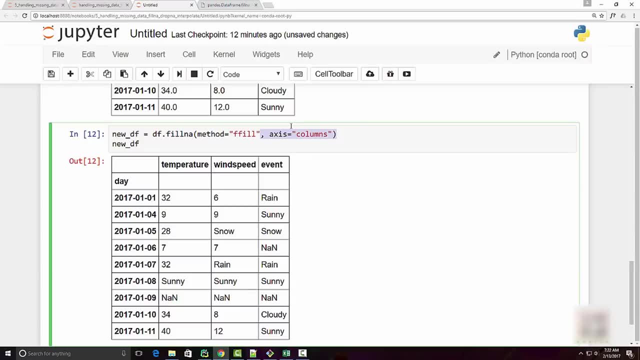 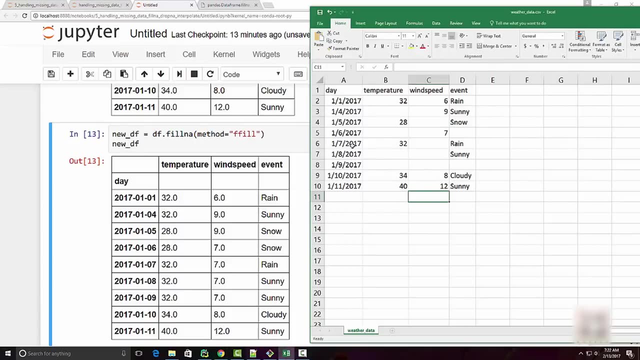 property or argument called limit. so let me show you what limit can do for you, okay. so here I'm going to replace this with forward fill and just kind of show you. so when you have forward fill, let's say, in the case of 7 January I had 32 and it- 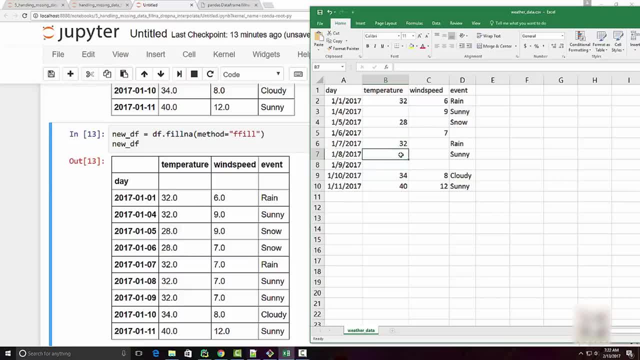 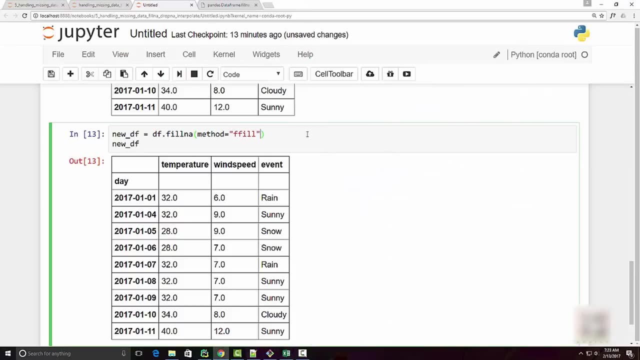 will just copy 32 to both of these missing data points. okay. now, let's say, due to some reason I want to carry forward this value only once. okay, so I want to copy it only here, but not here. in that case, you can specify limit and you can say: my limit is 1 as far as 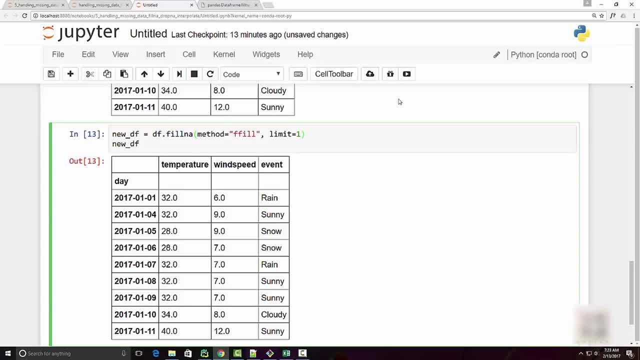 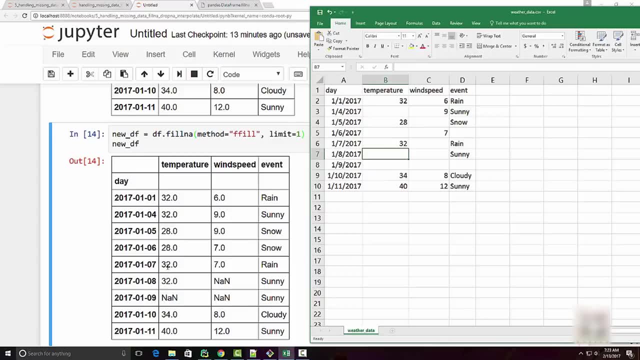 copying my valid value to missing value is concerned. okay, so when you run this you can see that now 7 January value was 32. it copied that to 8, but 9 still has any. because my limit is 1, I can copy it only once. okay, same thing here. 6. 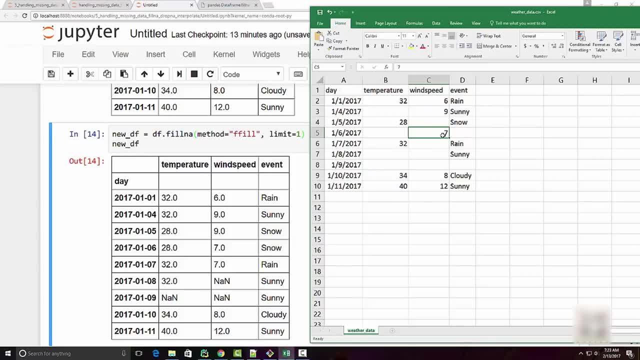 January wind speed was 7 miles per hour and it copied it to 7th, so you can see that 7 January now also has that value, but 8 and 9 January has any. okay, if you chain limit to be 2, you will notice that this 7 is copied here 2 times right: 7 and 7. 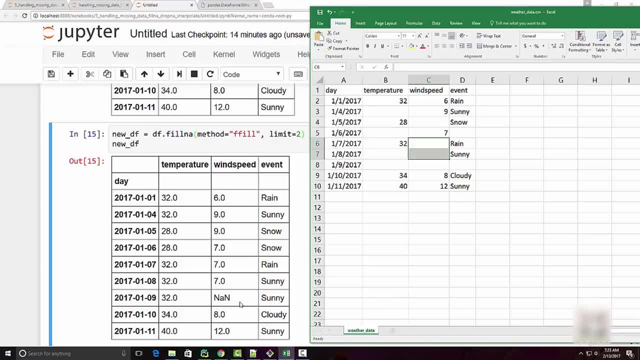 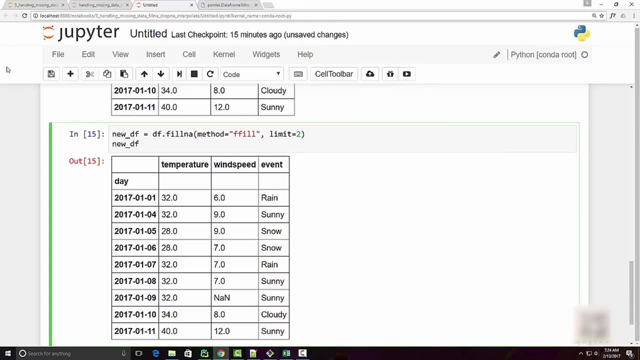 but my 9th January is still any okay. so this is how you can use your limit parameter. okay. now I'm still not happy with the guess that I'm making, because if the temperature on 1st January was 32 and on 5th it was 28, it is likely that 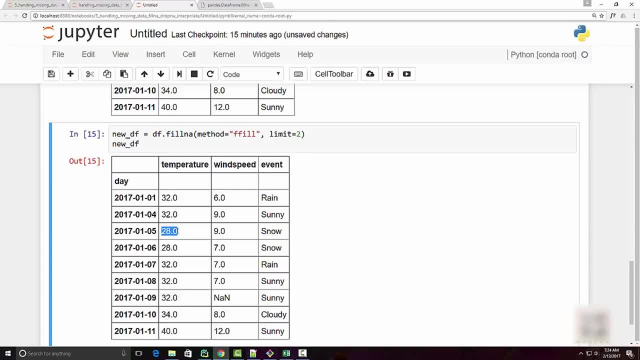 temperature on 4th was in between. okay, I mean, it's not always guaranteed, but that something you would consider to be correct. if you want to make sure that the consider a better guess, okay. so we have a method called interpolate in pandas. so let me just create a new cell and, by the way, I'm using the shortcuts you can you. 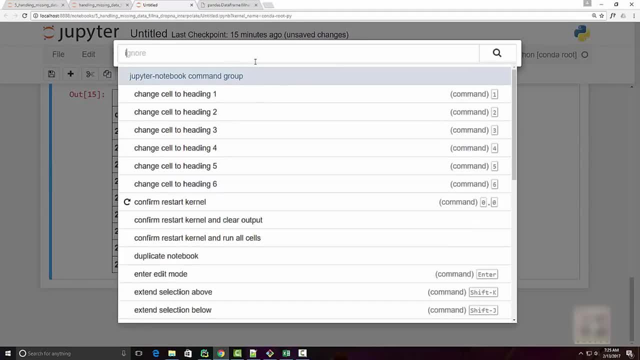 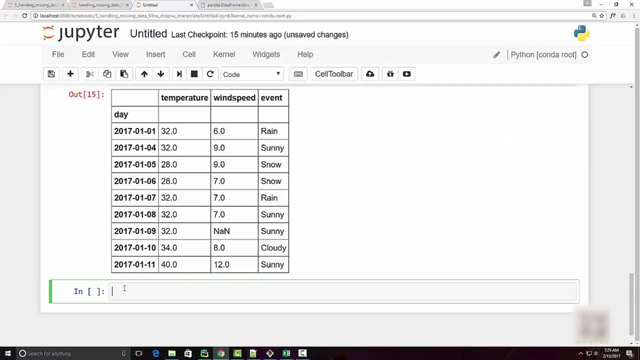 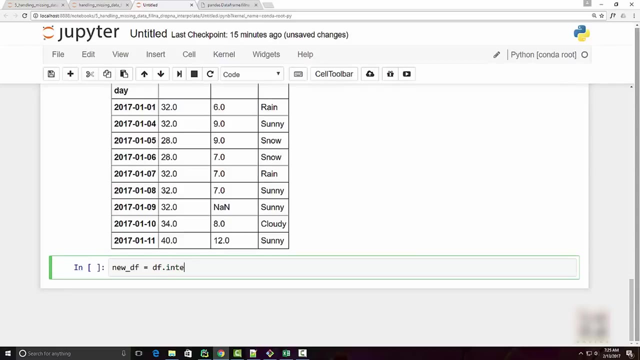 can you access all the shortcuts here? so when you say insert cell, below the shortcut is B. so that's what I'm using. so I'm here, I'm placing B. it's creating a new cell for me, okay. so here it's going to say dfinterpolate- okay. so when you do dfinterpolate, it's going to 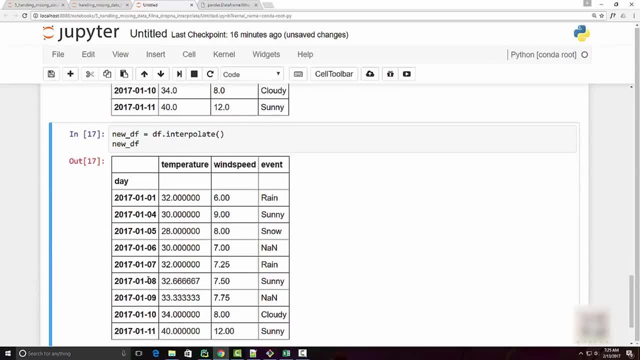 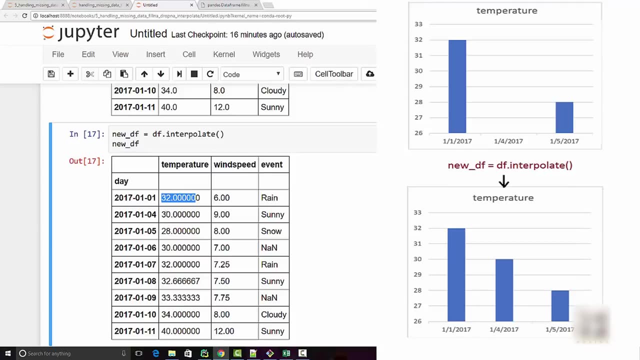 interpolate the values. so if you look at your new data from here, you will notice that now for the 4th January, it came up with a better guess, which is a linear interpolation. so if you have studied linear interpolation, you basically you will come up with this value 30, okay. so you just need to double check, okay. so now I am in the third. 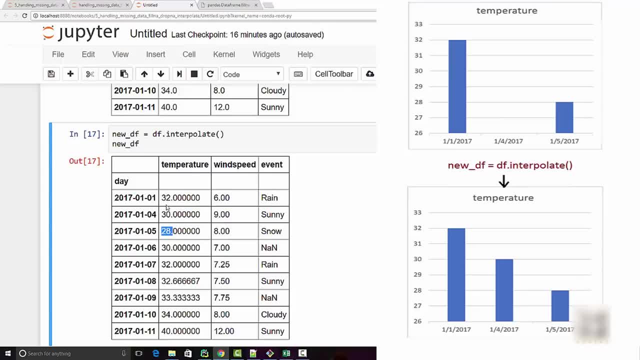 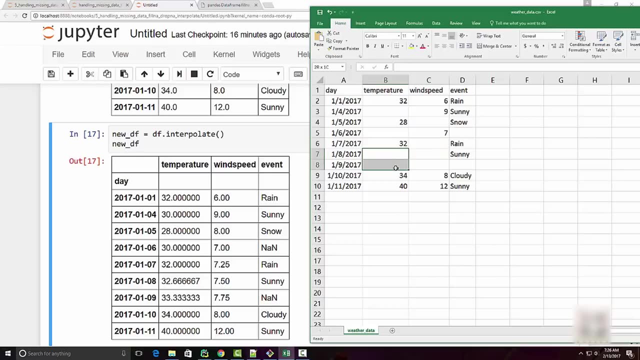 so it was 32- 28 and you're gradually transitioning and and having this intermediate data point. okay, so this is probably a better guess. okay, and it did the same thing for these two cells also. you can see that 32, 34 and here is 32. 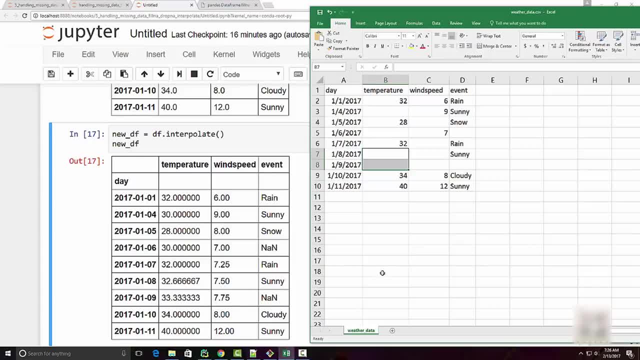 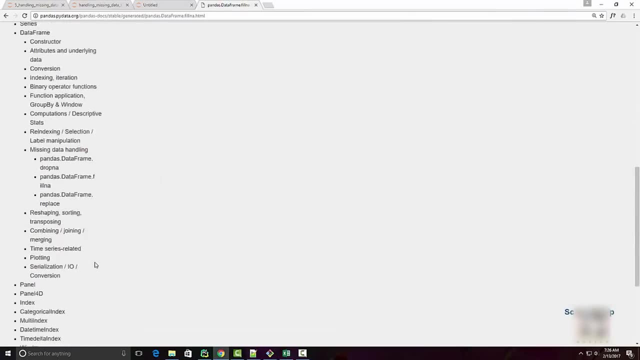 point 66, 33 point 33, so it's somehow coming up with this. it was 33 point of the tree, so it's using interpolation, linear interpolation, and coming up with this values. okay, so again, I'm going to go ahead and check the documentation for. 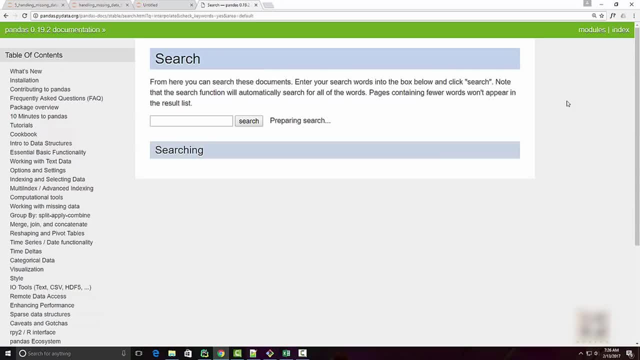 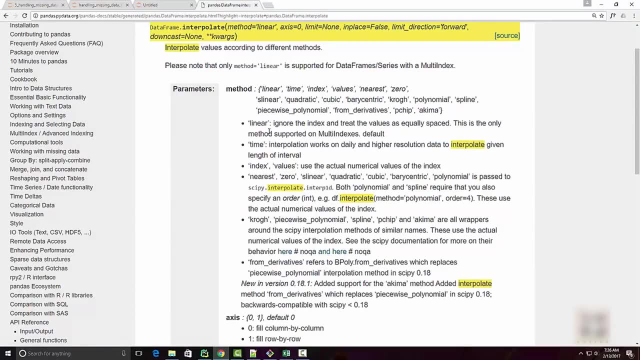 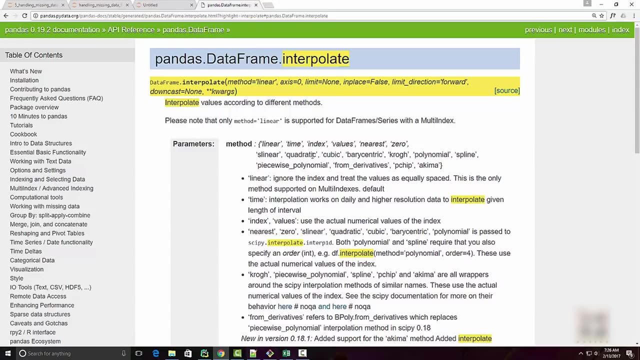 interpolate. so in search bar you can type in interpolate and look at data frame dot. interpolate documentation and you will notice that in a method if you don't specify anything, it is by default linear. but you can use so many other methods. you can use quadratic, cubic and piecewise polynomial. there are. 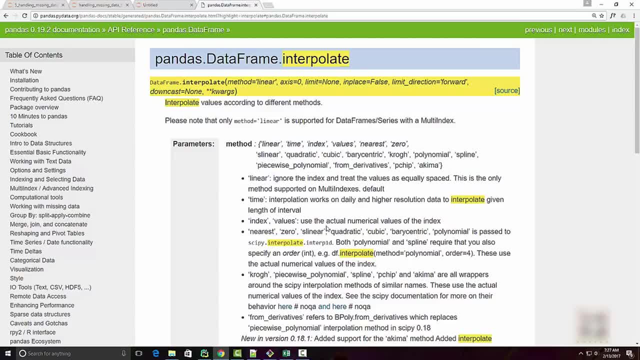 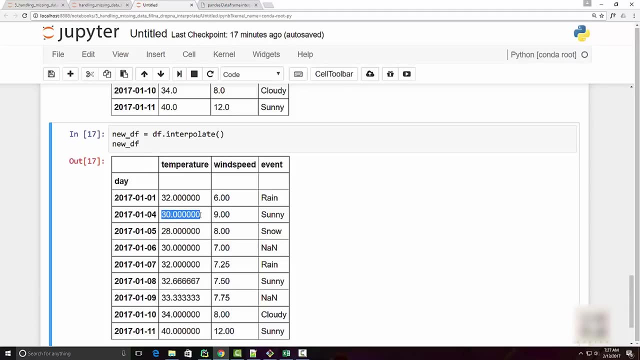 so many methods to specify as far as your interpolation is concerned. okay, so I'm going to use time now, so let's see what time can do for us. so here, before we do that, you will see that using linear interpolation it came up with the middle value, okay, 32 and 28. the middle value is 30, but look at the date, okay. 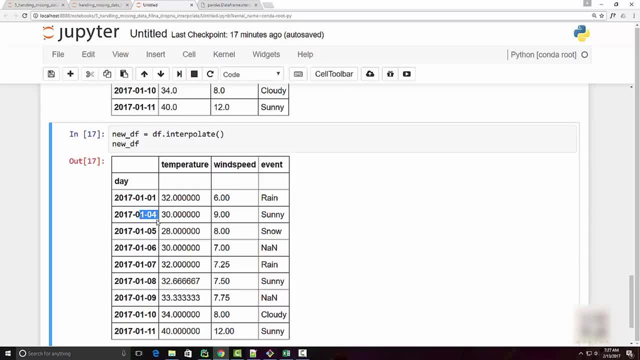 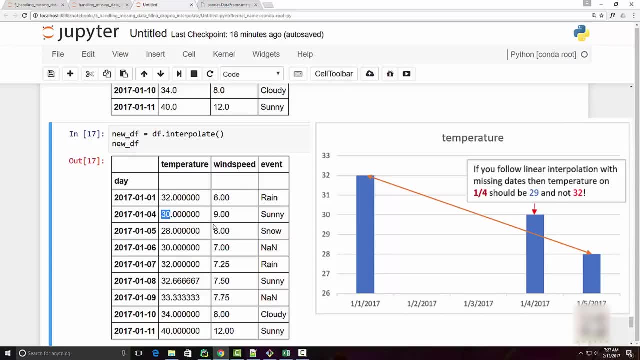 date is not in the middle. okay. date is more near towards 5th January. okay, so I'm missing 2nd and 3rd January. so 30 still doesn't look like a better guess. it should be relatively near to this value, 28. so when you use method equal to time. 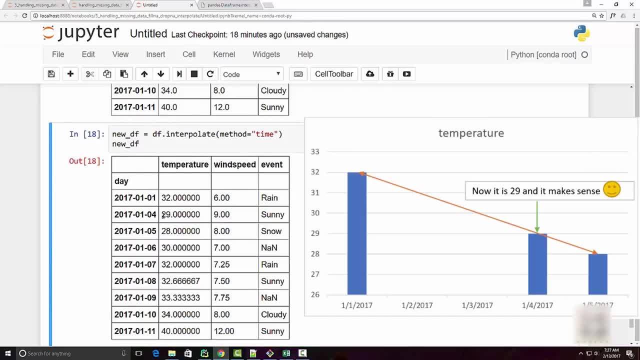 you can see that now it came up with value 29 because now it is considering this time, this date. also, in coming up with this value, it is realizing that 4th January is near to 5th, hence the value should not be excellent middle, but it. 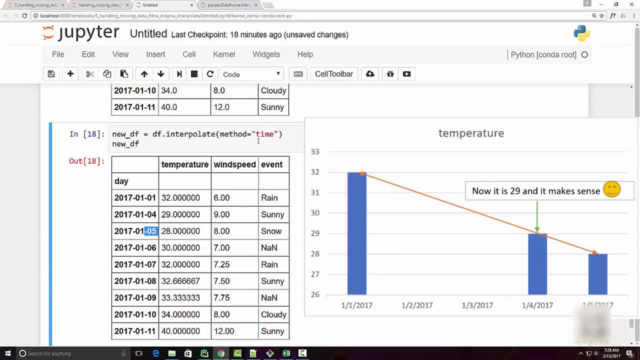 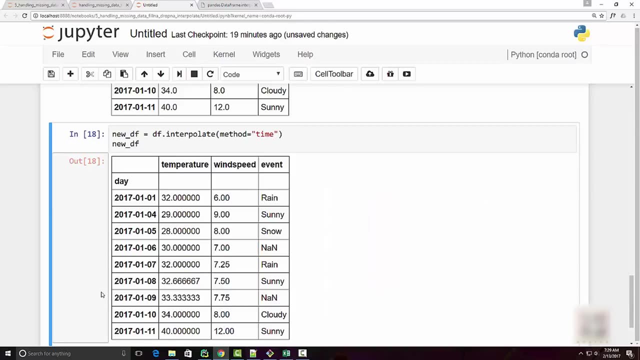 should be more near to this value. okay, so this feature I found to be pretty powerful whenever you are making a guess or estimate for missing values. okay, so far, so good. sometimes, based on the situation, I just want to, let's say, drop all the rows with any values in. 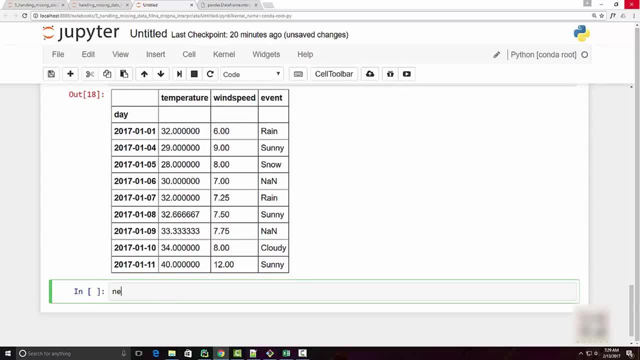 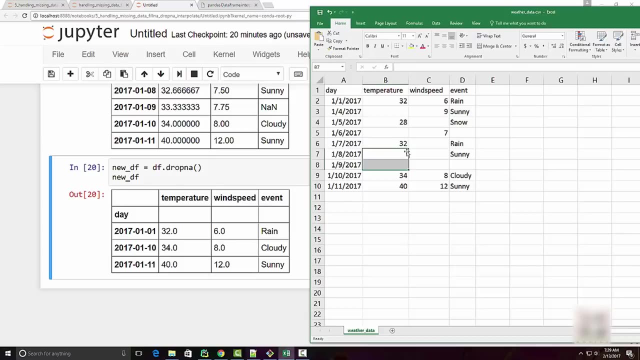 that case you can use this method called drop any. you can say DF, drop any, okay, and Gripen printing the new data frame. so you can see that in my excel sheet, whichever row had any any value, okay, it dropped all of them. so now I got only three rows, which has a valid. 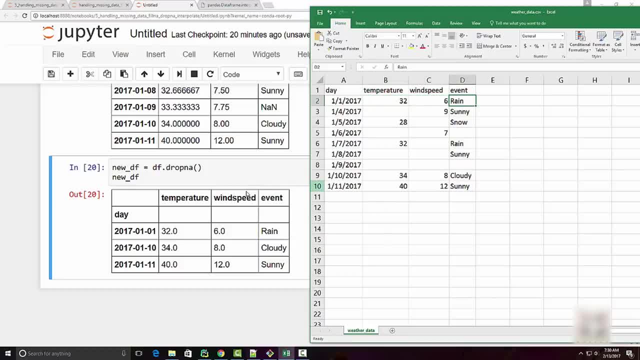 content in all of the columns. okay, sometimes you want to drop the row if it has at least one any. okay, so here, what it is doing is actually it is doing that. so here, if you have at least one any, it is dropping it. but let's say I want to. 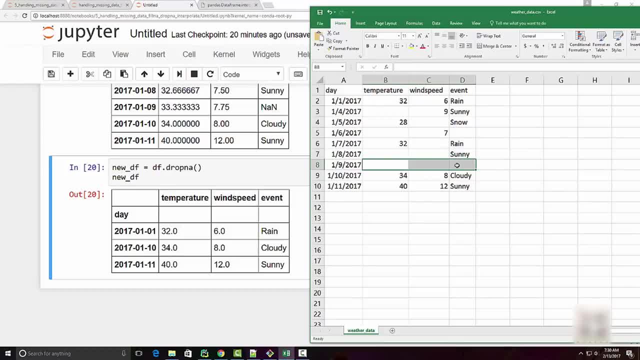 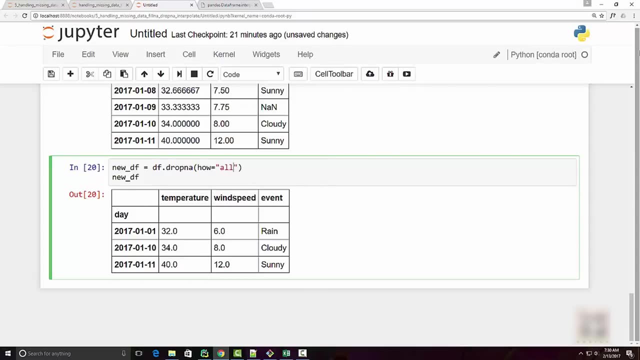 drop only if it has all any. so, for example, I want to drop this row, but I still want to preserve these rows because it has at least some data. okay, so for that you can use how parameter. you can say: how is equal to all. so now you don't see 9th January here in this data. 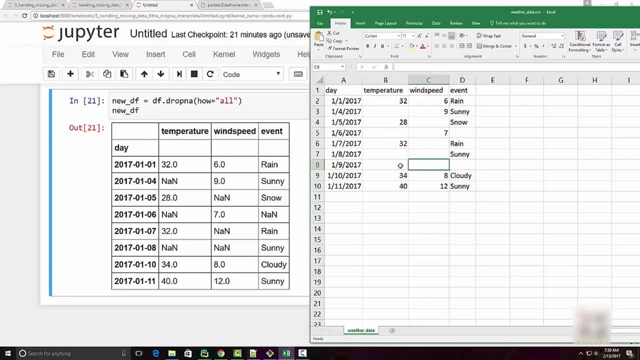 frame, but you can see that it has at least one, any. so here, what it is doing is it is not considering any value, because it had all the values to be any. it has this date, but this date is a index, so it is not considering. it is not considering. 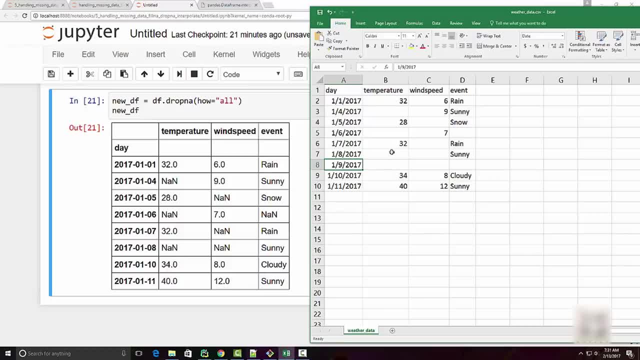 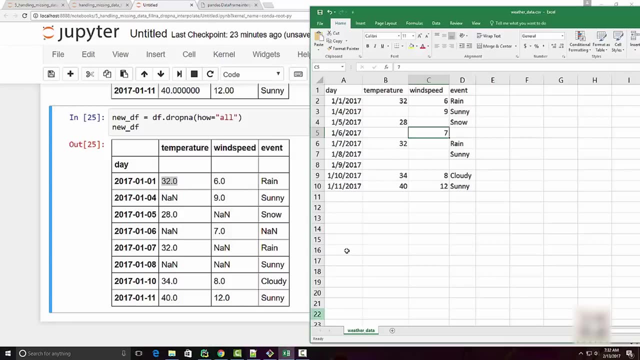 that in in the process of dropping, okay, and these values, these rows, has some any cells, but not everything is any. so it's not dropping that, okay. now what if I want to go by non, any value? so let's say I want to say that if I have at least one, 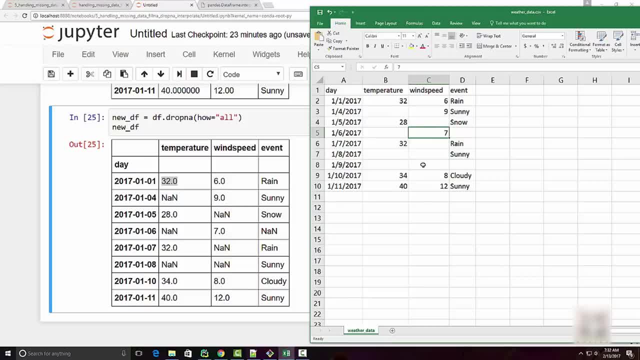 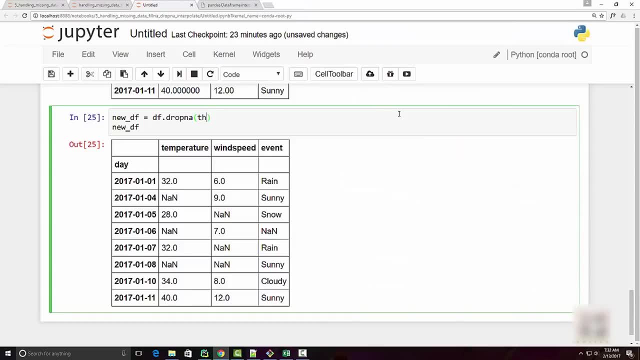 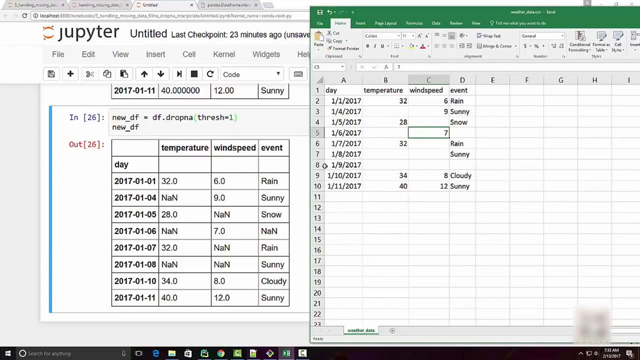 non any value, then keep that row and drop any other rows. so for that you can use a threshold parameter so you can say threshold equal to one. threshold equal to one means if I have at least one non any value, then keep the row. okay. so when you run that see what happens is again the same result. 9th January got dropped. 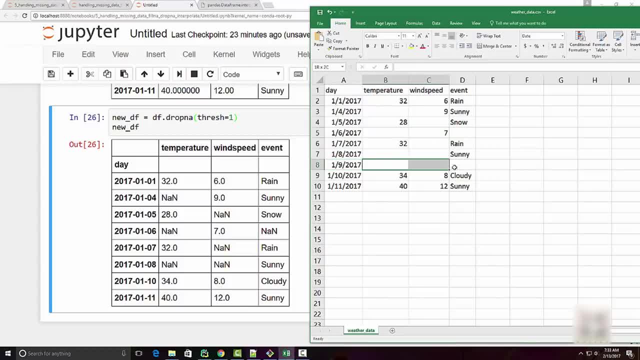 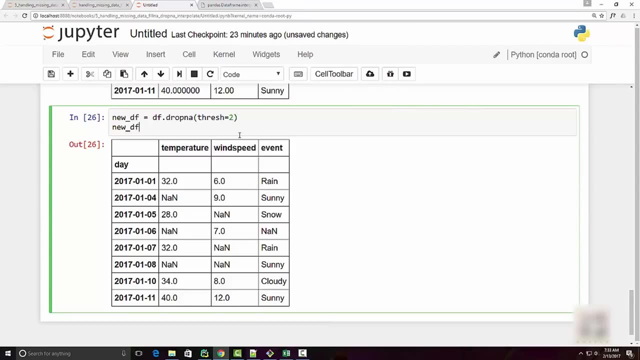 because it doesn't have any valid value. everything was any okay, now let's. so. it kept this 6th January value because it has at least one valid value. so if I change threshold to be one, what it means is: alright, so let's run this. okay now, when I say threshold equal to two, it dropped this. 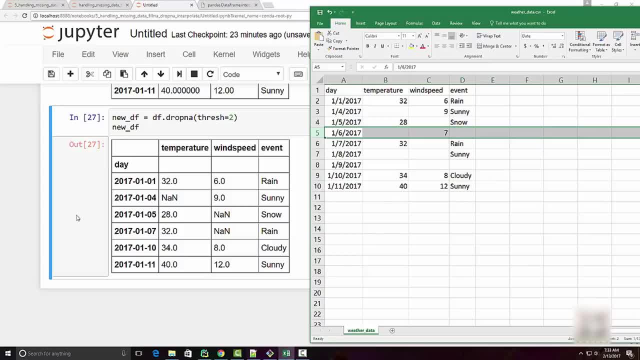 particular. you can see it dropped that particular row because two means I need two valid values in order to keep the row, but I don't have two valid values. I have only one value. the date is not counted because it is index. okay, so if I have one value, I'm going to drop it. okay, so 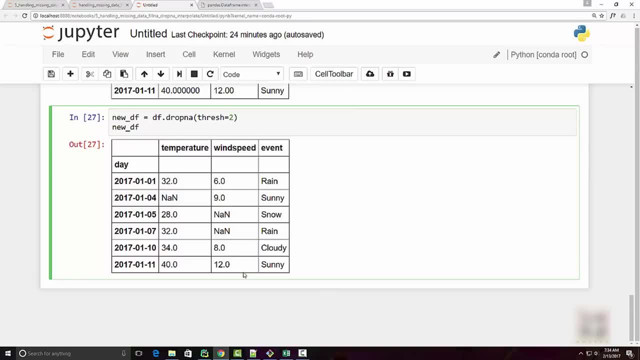 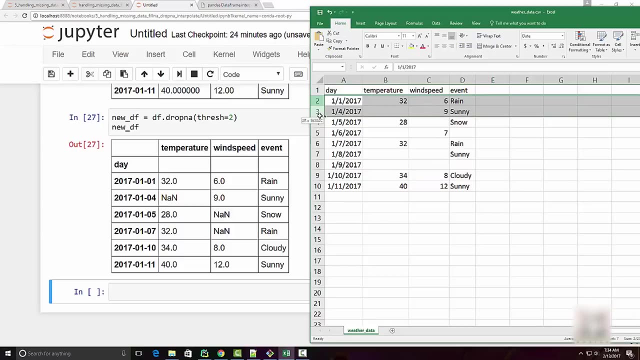 you can use threshold to drive your dropping process by number of valid values that you have. okay, last thing that we want to cover is: how do you go about inserting the missing date? so I don't have second and third January here. I want to, let's say, insert those dates. so for that you will do something like: 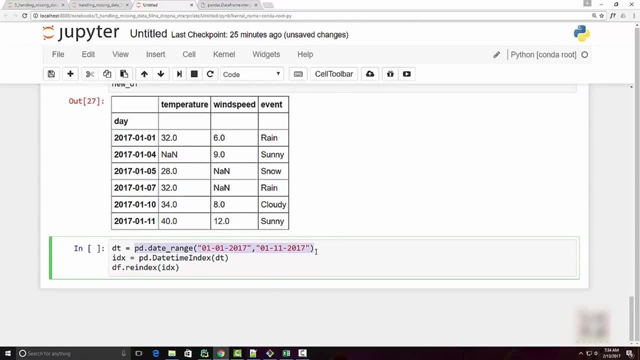 this. so here you will create a date range and using the date range. so let's say, I have a date range from 1st January to 11 January. so 1st January to 11 January I created a date range. so this is your date range and you pass that to. 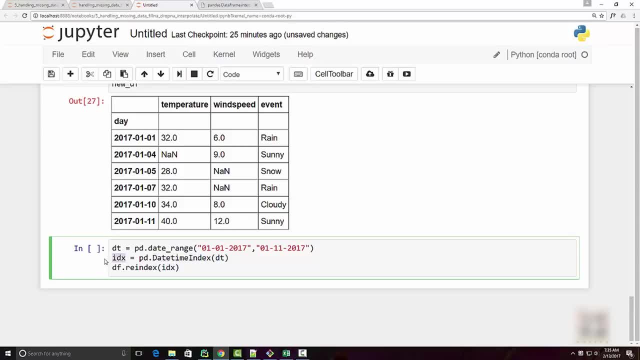 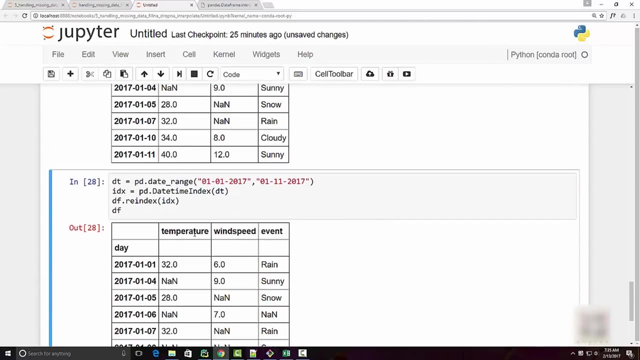 date time index and create a date time index and then you do reindex in your data frame. so I'm saying DF dot reindex using that index and then you print your data frame again. so you have to do in place equal to true. okay, I'm.